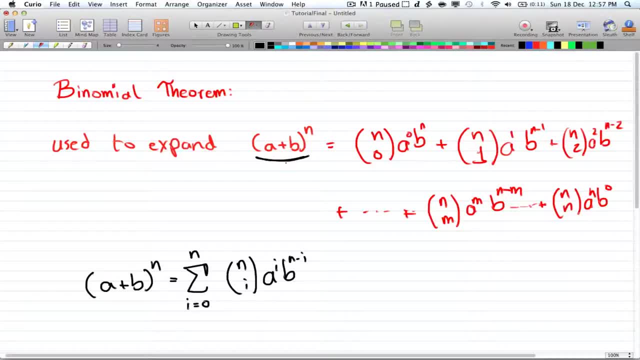 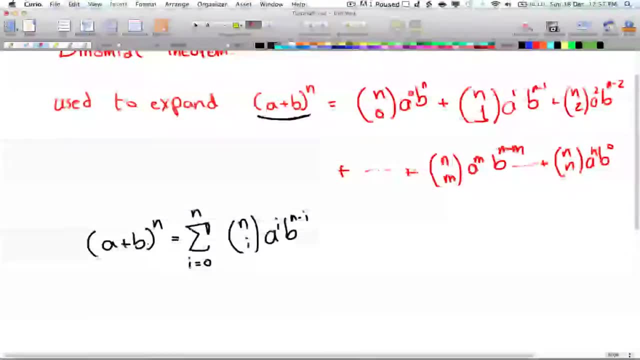 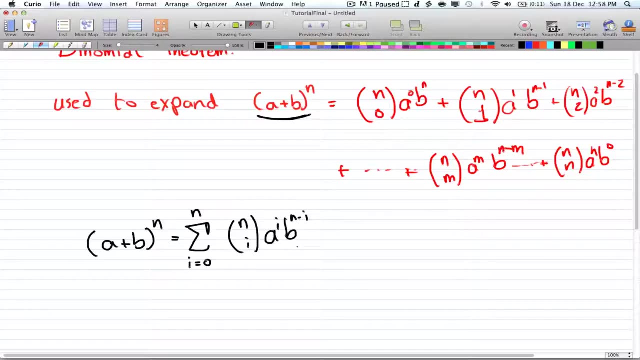 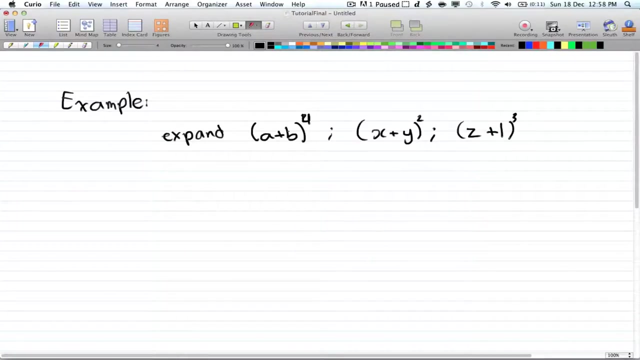 So this is used as a simple way of evaluating any term in this form here, And this is the shorthand formula for it, And you really have to know this. Just know the 4, the way to represent it, And here are a few examples. So if you want to expand a plus b to the power of 4.. So let's take it. 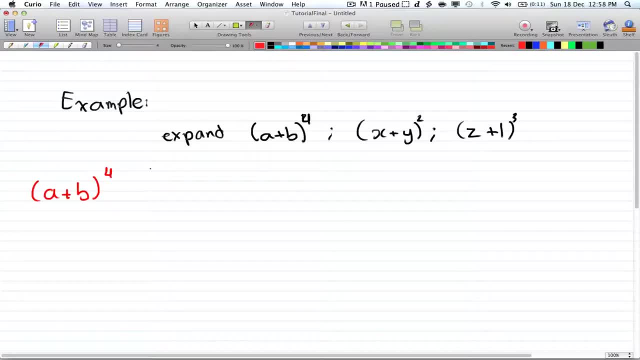 a plus b to the fourth And our formula is: the sum of i is equal to 0 to n and our n here is equal to 4, of n choose i, So n choose. let's put 4 there. 4 choose i times a to the power of i. 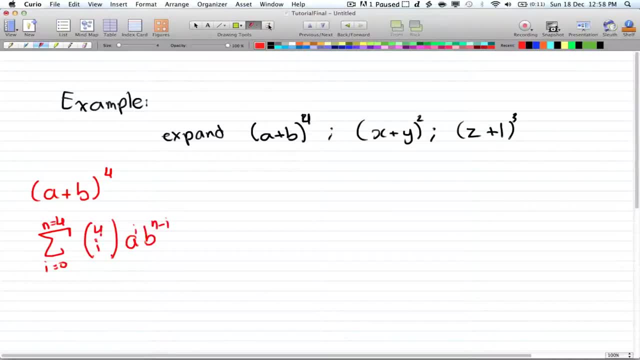 a times b to the power of n minus i, So 4 minus 1.. Or 4 minus i, rather, So 4 minus i, And by expanding this you're going to get 4. choose 0 of b to the fourth plus 4. choose 1 of a times b to the third plus 4. choose 2 of a to the. 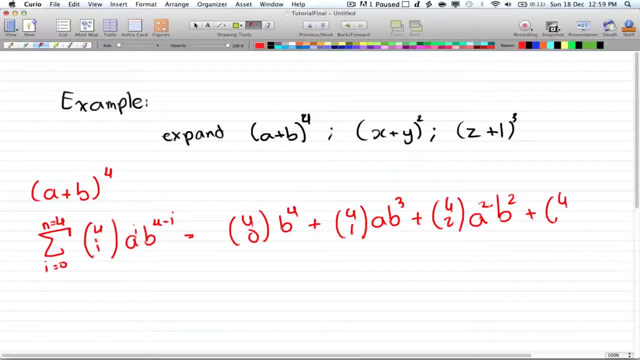 second and b to the second plus 4. choose 3 of a to the third and b plus 4, choose 4 times a, And here a is to the power of 0, so it's equal to 1.. 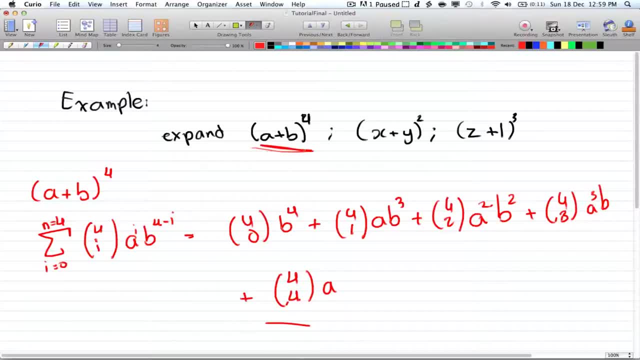 And this is your answer for expanding this term here. Okay, so for the second part, all we have to do is change our n so we get 2, so that is n, And our a is going to be equal to x and our y is going to be equal to b. 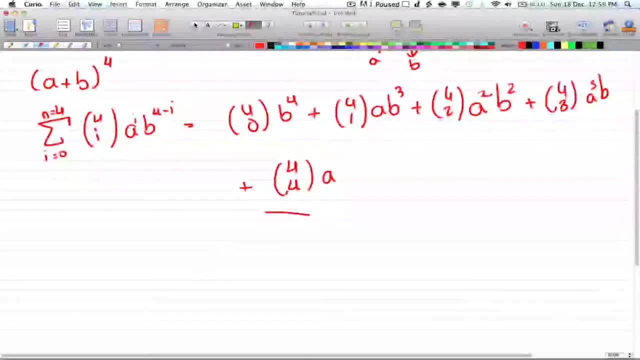 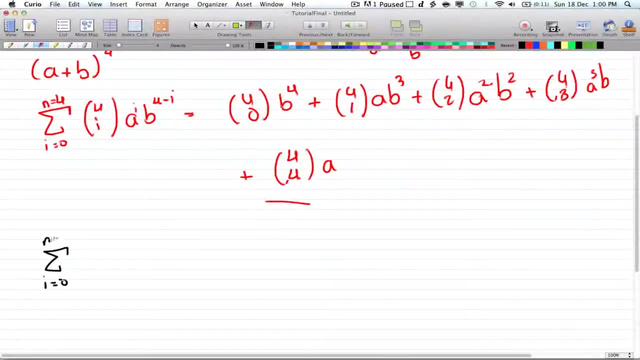 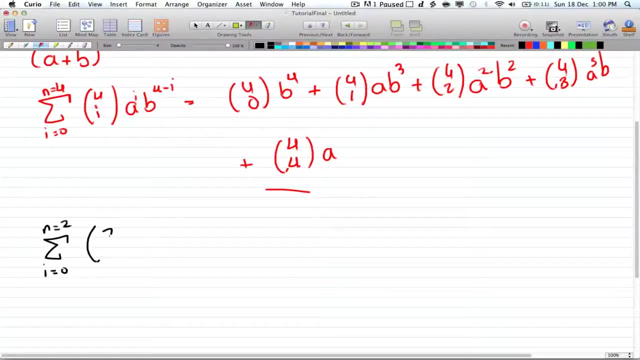 So by just replacing the variables in our formula you can get. So let's see: The sum of i is equal to 0,, n is equal to 2.. You can see, here we have 2. And then you have n. choose i, which is 2, choose 1, times a to the power of. 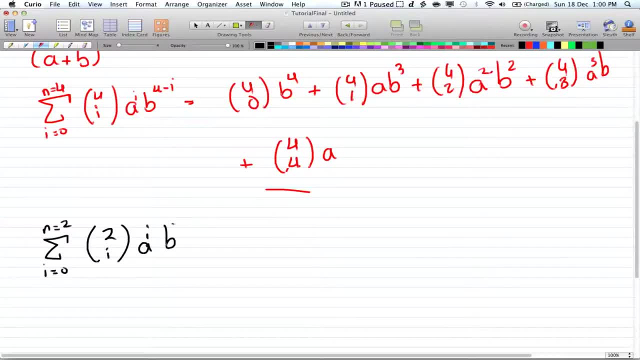 n minus i times b to the power of n minus i, And in this case our a is x and our b is y. So let's just go ahead and replace them so x and y, And that will be equal to 2. choose 0 of x to the power of 0 and y to the power of 2,. 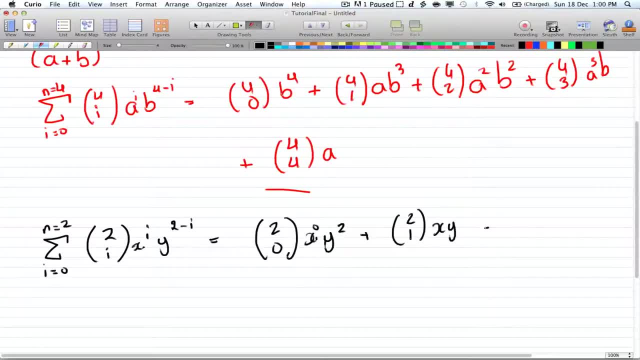 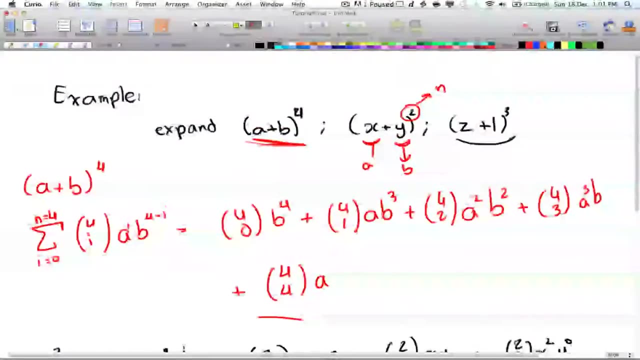 plus 2. choose 1 of x times y plus 2. choose 2 of x squared times y to the power of 0. And that's our result here. Our last example is going to be z plus 1 cubed. We have z plus 1 cubed. 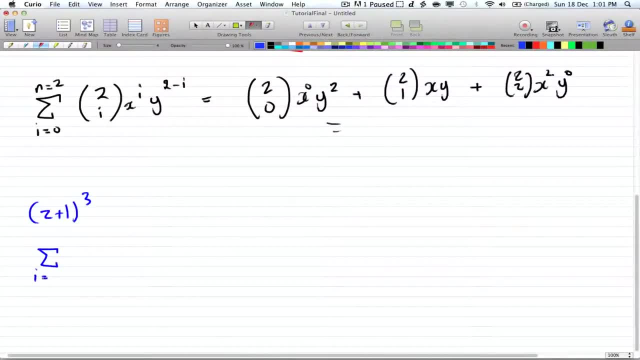 Again. we'll just use the formula to get: i is equal to 0, and n is equal to 3.. So there's our n once again, And in this case our a is going to be z and our b is going to be 1.. 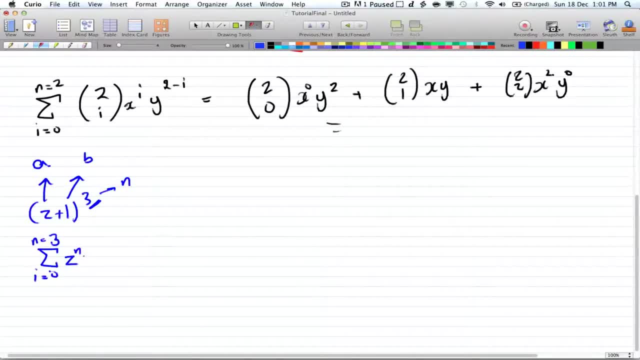 So we have z to the power of i times 1 to the power of n minus i. This is going to be equal to: By expanding this term here you'll get 3 choose 0.. I actually forgot to include the choose term. 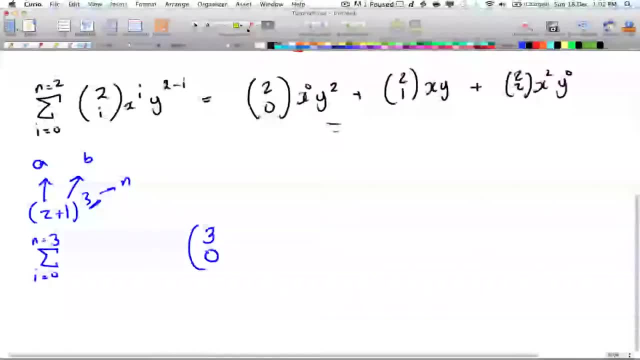 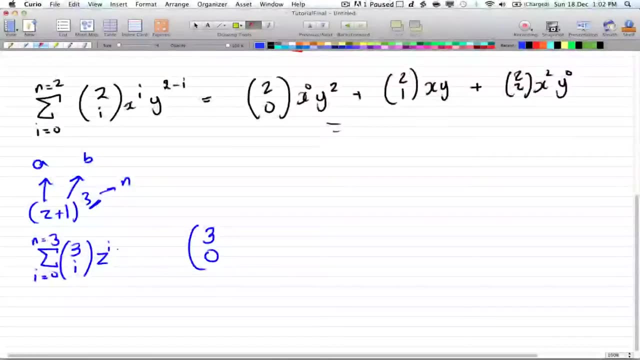 Okay, whatever, I'll just rewrite it again. So you have 3. choose i of z to the power of i times 1 to the power of n minus i. So you have 3. choose 0 and z to the power of 0 times 1 to the power of 3,. 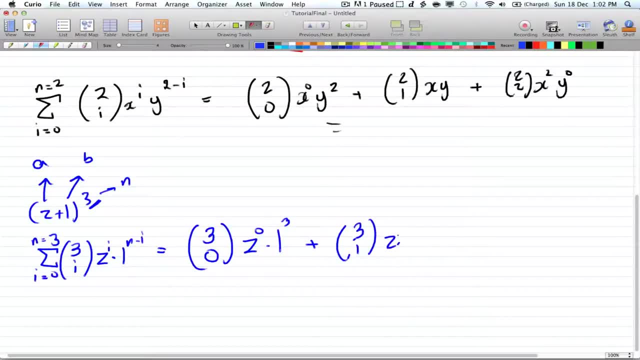 plus 3 to the power of 1 times z, to the power of 1 times 1 squared, And the 1s don't really count, so you don't even have to write them. So, plus 3, choose 2 z squared. 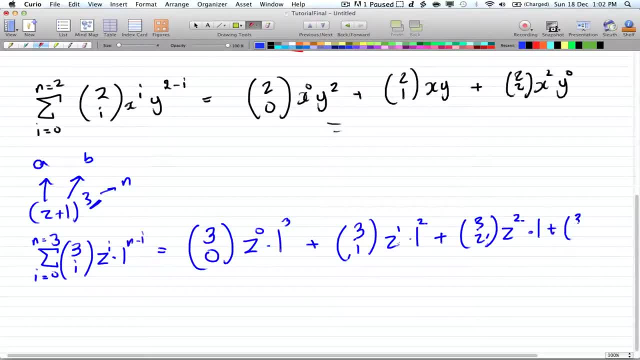 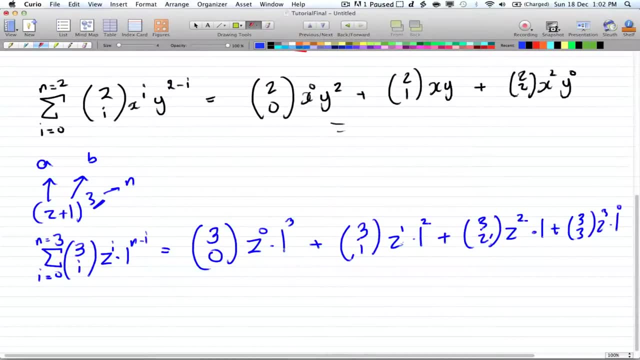 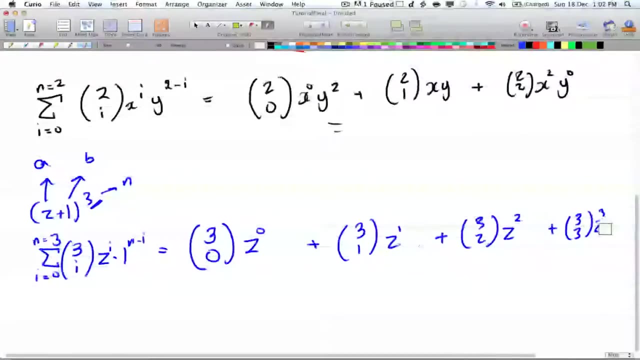 times 1 plus 3, choose 3 of z cubed times 1 to the power of 0., And whenever you have this form here where it's only one term, so let's just cancel out the 1s You have z. 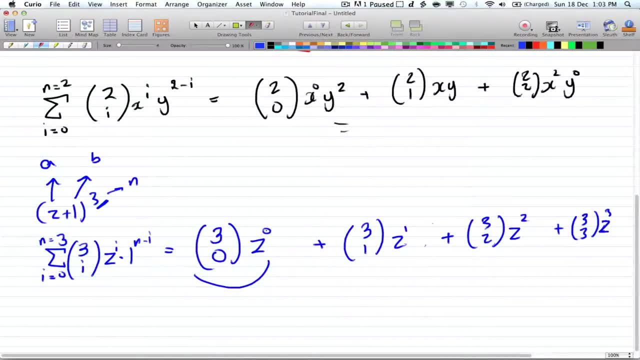 So whenever you have this form here where it's like z to the power of 0,, z to the power of 1, and there's no second term, so the b term is missing, then this will become: you take whatever a is, so a plus 1 to the power of n. 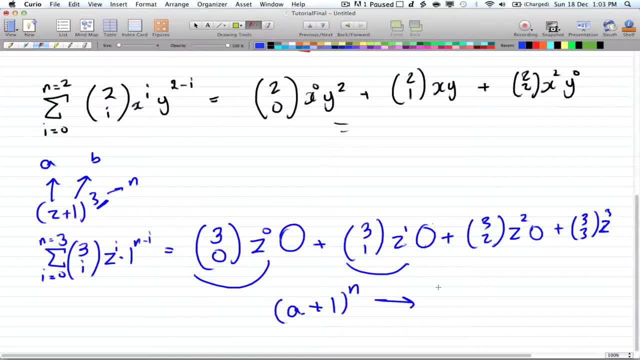 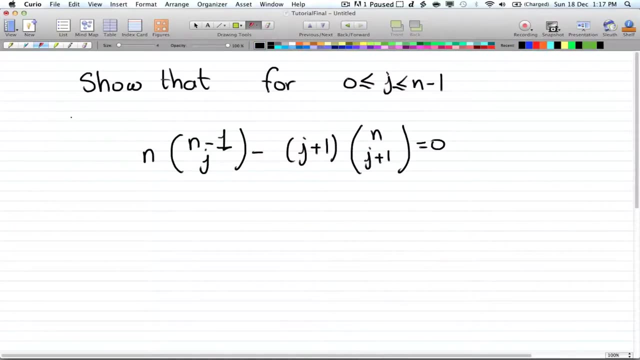 where n is the term you're choosing. So in this case it's going to be z plus 1, choose 3.. You're going to have to convert it both ways, So you should know how to get to this form here. Alright, so here we have a combination problem. 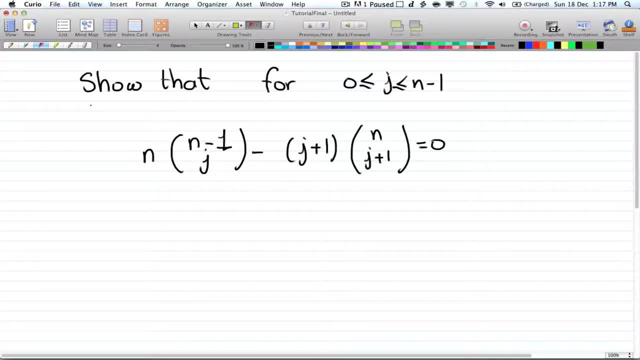 And we have to show that for 0 smaller than or equal to j is smaller than or equal to n minus 1, you have n times n minus 1. choose j minus j plus 1. times n. choose j plus 1.. 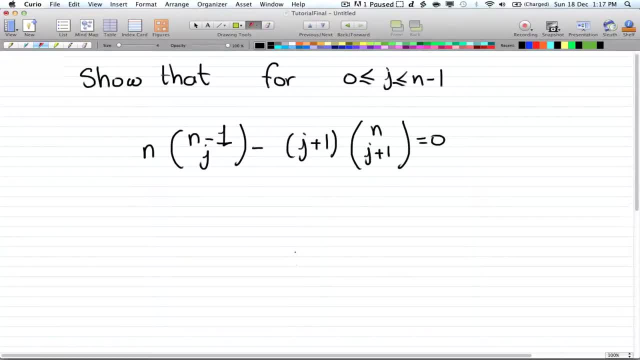 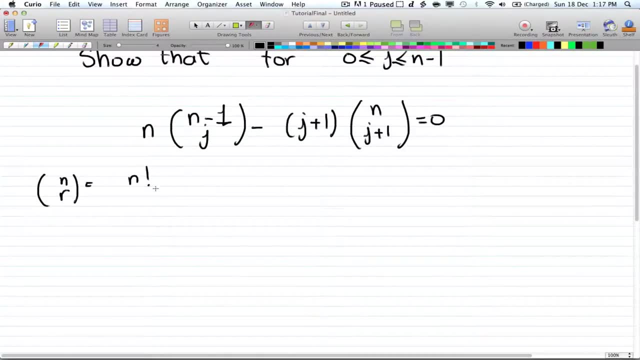 We have to show that this here is equal to 0. So remember that for any term n choose, r is equal to n factorial 0. Over r factorial times, n minus r factorial. So the first thing you have to do is expand this term here. 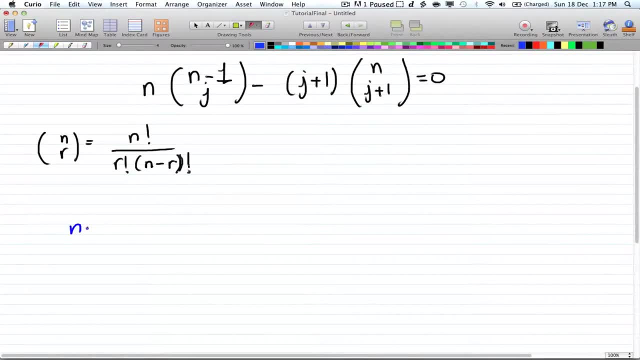 So you'll get n times n minus 1 factorial, n minus 1 factorial divided by j factorial times j factorial times n minus 1 minus j factorial, And then subtract j plus 1, multiplied by the second term. here now.